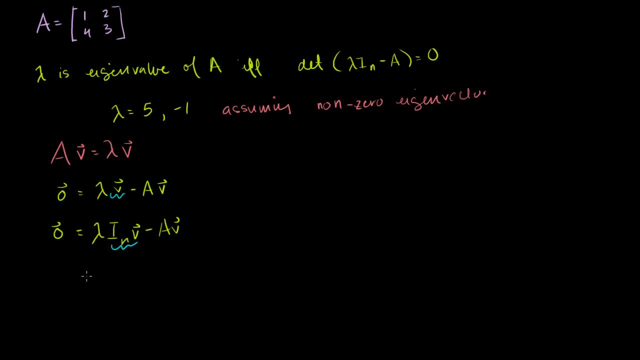 Then you factor out the V, so to speak, because we know that matrix vector products exhibit the distributive property And we get lambda times the identity matrix minus A times my eigenvector have got to be equal to 0. Or another way to say it is for any lambda eigenvalue, let me 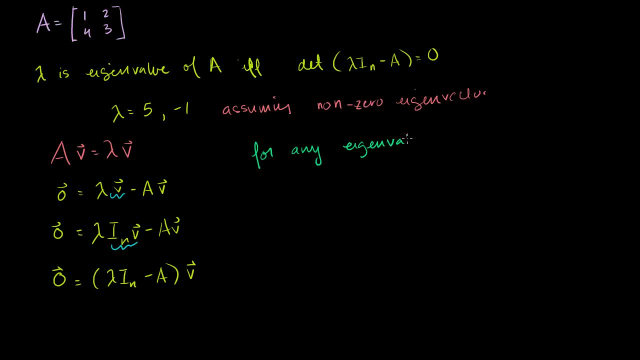 write it for any eigenvalue- lambda- the eigenvectors that correspond to that lambda. we can call that the eigenspace, The eigenspace for lambda. So that's a new word: Eigenspace. Eigenspace just means all of the eigenvectors that. 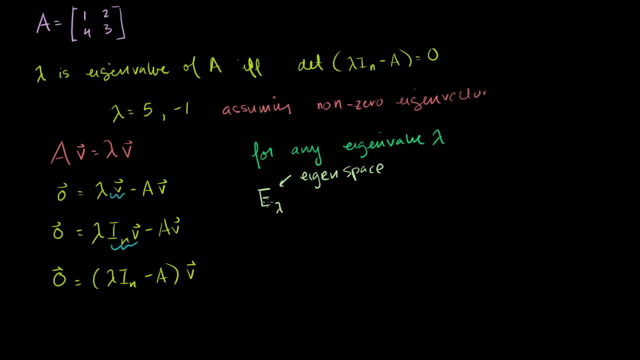 correspond to some eigenvalue. The eigenspace for that, for some particular eigenvalue, is going to be equal to the set of vectors that satisfy this equation. Well, the set of vectors that satisfy this equation is just the null space of that, right there. 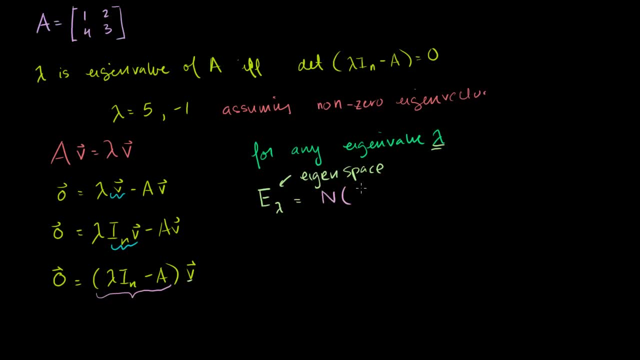 So it's equal to. It's equal to the null space of this matrix right there, The null space matrix of lambda times the identity matrix, and by an identity matrix minus A. And so everything I've done here, this is true. 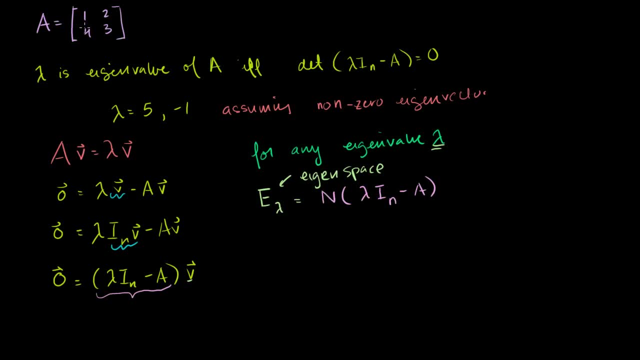 This is the general case, But now we can apply this notion to this matrix A right here. So we know that 5 is an eigenvalue. So for, let's say for lambda is equal to 5.. The eigenspace that corresponds to 5 is equal to. 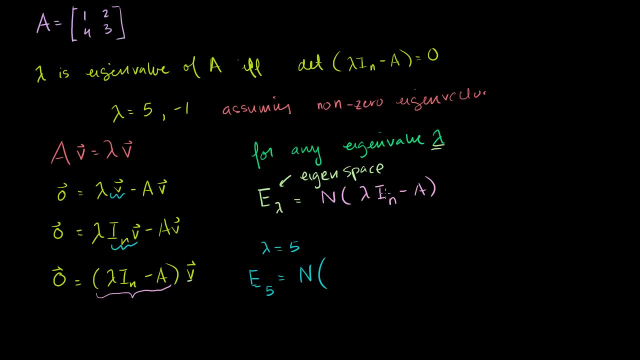 the null space of. well, what is 5 times the identity matrix? 5 is going to be the 2 by 2 identity matrix, right, 5 times the identity matrix is just 5, 0, 0, 5.. 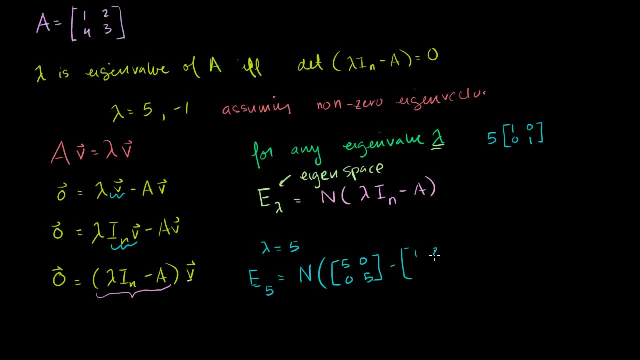 Minus A, That's just 1,, 2, 4, 3.. So that is equal to the null space of the matrix. 5 minus 1 is 4.. 0 minus 2 is minus 2.. 0 minus 4 is minus 4.. 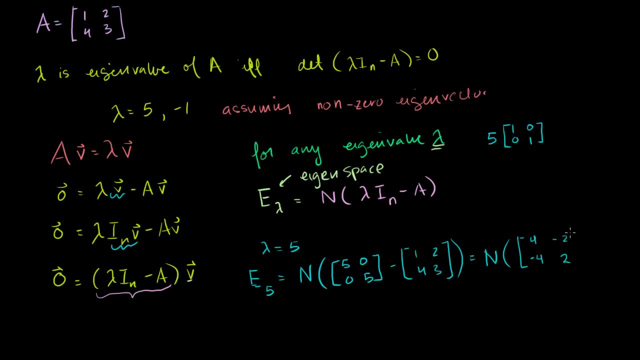 And then 5 minus 3 is 2.. So the null space of this matrix right here- and this matrix is just an actual numerical representation of this matrix right here, The null space of this matrix is the set of all of the vectors that satisfy this, or all of the eigenvectors that. 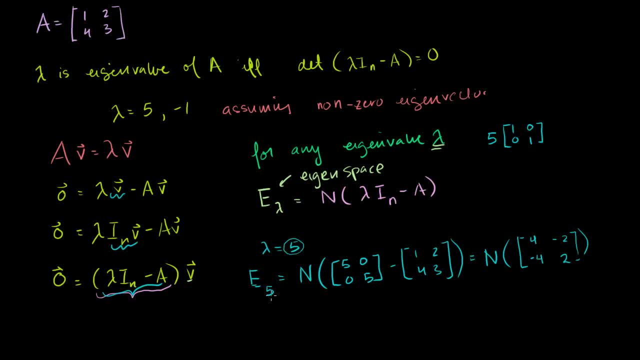 correspond to this eigenvalue. Thank you, Bye, Bye, Bye you. or the eigenspace that corresponds to the eigenvalue 5.. These are all equivalent statements, So we just need to figure out. the null space of this guy is. 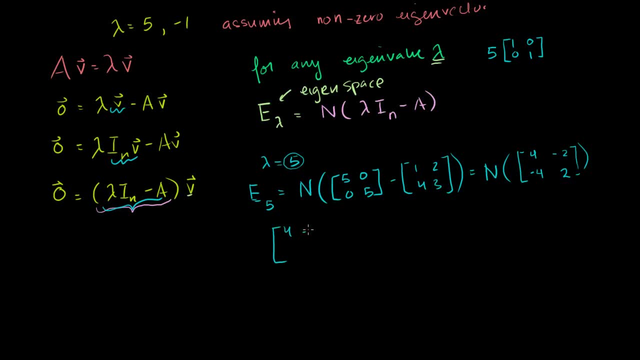 all the vectors that satisfy the equation 4 minus 2 minus 4, 2 times some eigenvector is equal to the 0 vector And the null space of a matrix is equal to the null space of the reduced row. echelon form of a matrix. 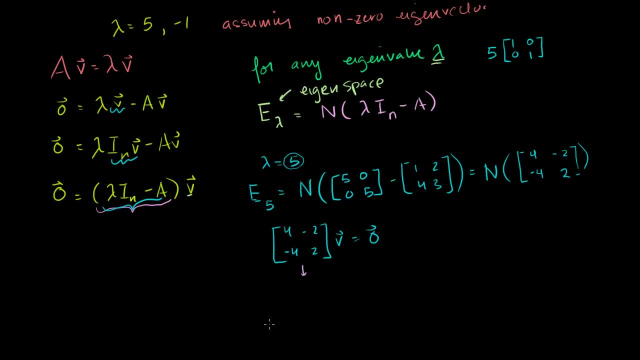 So what's the reduced row echelon form of this guy? Well, that's, I guess, a good starting point. Let me keep my first row the same: 4 minus 2.. And let me replace my second row with my second row plus my. 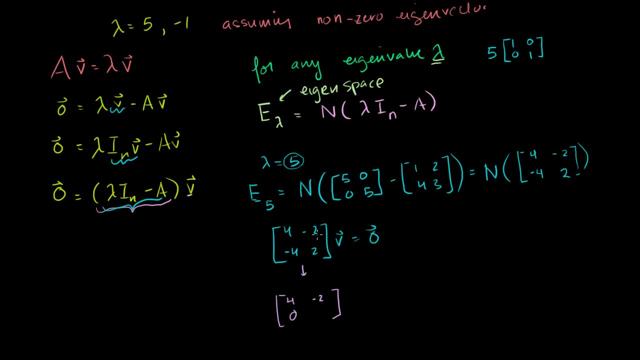 first row. So minus 4 plus 4 is 0.. 2 plus minus 2 is 0.. Now let me divide my first row by 4, and I get 1 minus 1 half, and then I get 0, 0.. 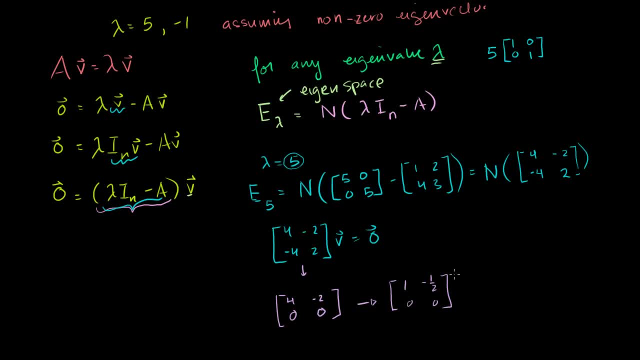 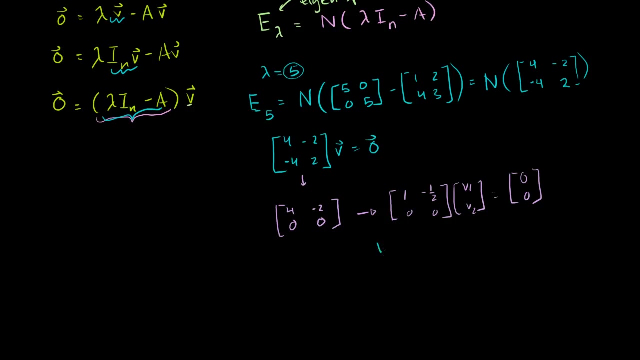 So what's the null space of this? This corresponds to v, This times v1, v2.. That's just another way of writing. my eigenvector, v, has got to be equal to the 0 vector, Or another way to say it is that my first entry, v1, which 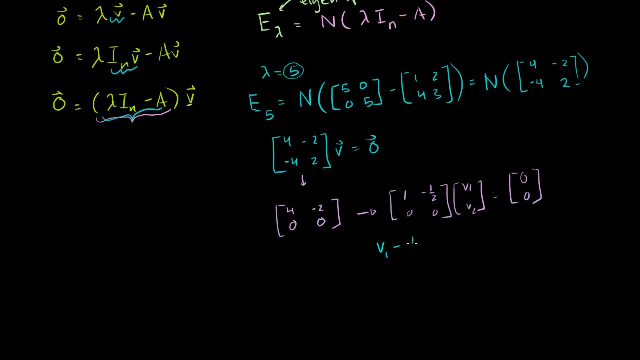 corresponds to this pivot column plus or minus 1 half times. my second entry has got to be equal to that 0, right there. or v1 is equal to 1 half v2.. And so if I wanted to write all of the eigenvectors that, 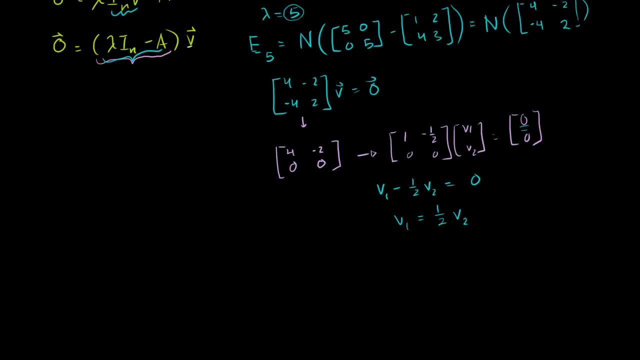 satisfy this. so I could write it this way: My eigenspace, that corresponds to lambda, equals 5,. that corresponds to the eigenvalue 5, is equal to the set of all of the vectors v1,, v2 that are equal to some scaling factor. 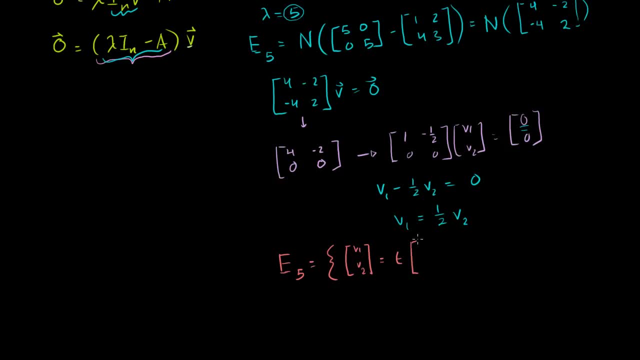 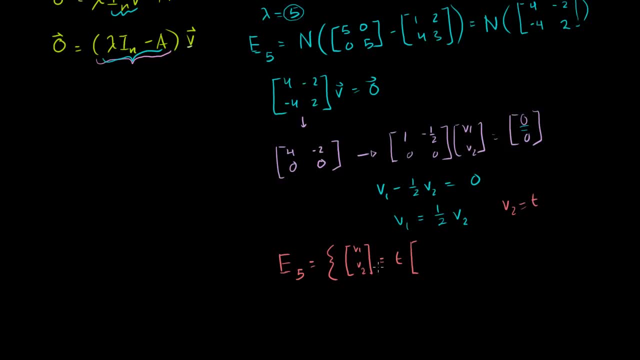 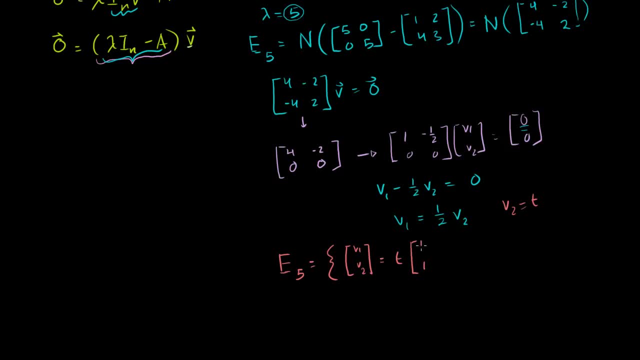 to be equal to 1 half times v2, or 1 half times t, 1 half times t, just like that, for any t is a member of the real numbers And, if we wanted to, we could scale this up. 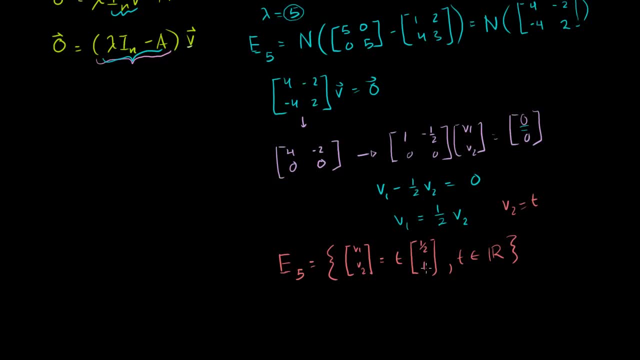 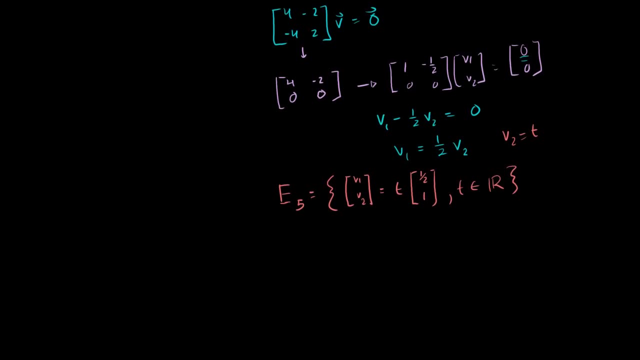 We could say any real number times 1, 2.. That would also be the span. Let me do that actually. It'll make it a little bit cleaner. Actually I don't have to do that. So we could write that the eigenspace for the eigenvalue 5. 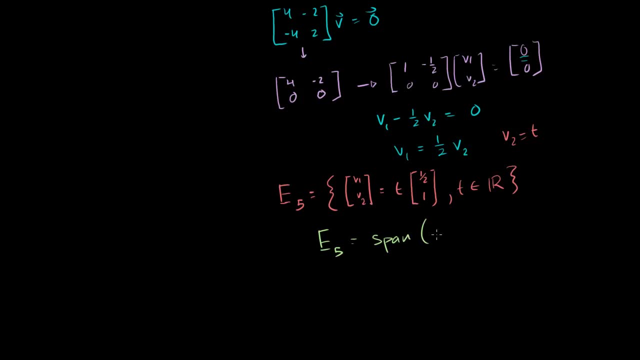 is equal to the span of the vector 1, half and 1.. So it's a line in R2.. Those are all of the eigenvectors that work for the equation where the eigenvalue is equal to 5.. Now what about when the eigenvalue is equal to 1?? 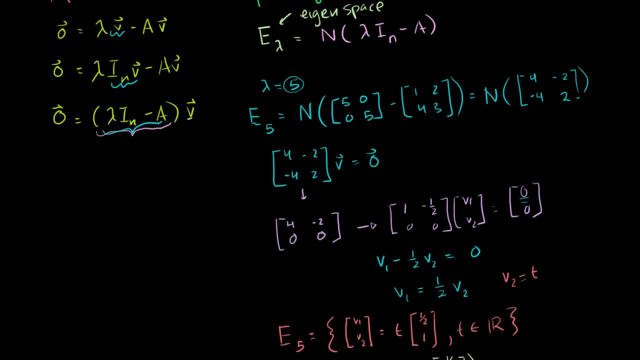 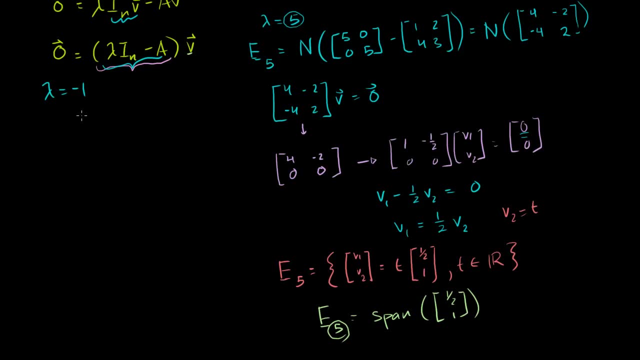 When the eigenvalue is equal to minus 1, so let's do that case. When lambda is equal to minus 1, then it's going to be the null space. So the eigenspace for lambda is equal to minus 1 is going to. 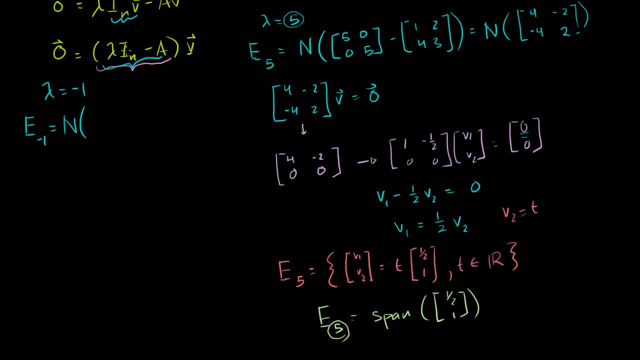 be the null space of lambda times, our identity matrix, which is going to be minus 1, 0, 0, minus 1.. It's going to be minus 1 times 1, 0, 0, 1, which is just minus. 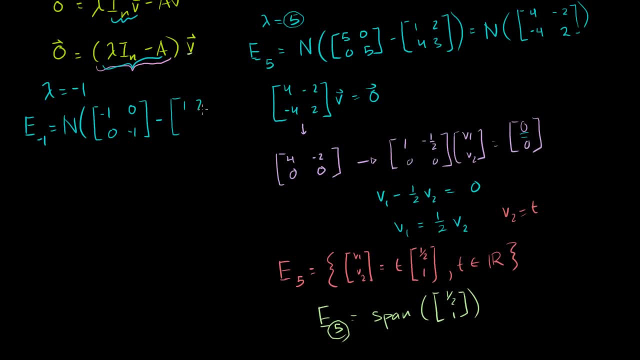 1 there minus a, so minus 1,, 2,, 4, 3.. And this is equal to the null space of minus 1, minus 1 is minus 2, 0, minus 2 is minus 2, 0, minus 4 is minus 4, and. 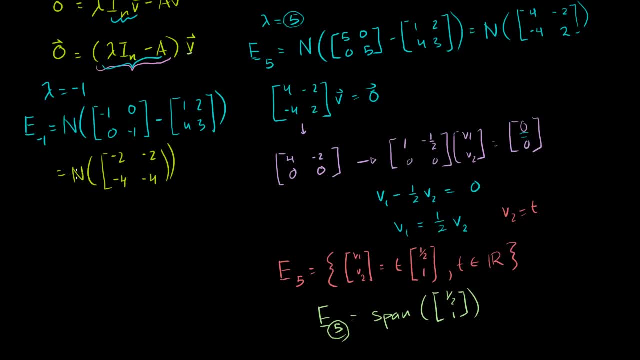 minus 1, minus 3 is minus 4.. And that's going to be equal to the null space of the reduced row echelon form of that, So we can perform some row operations right here. Let me just put it in reduced row echelon form. 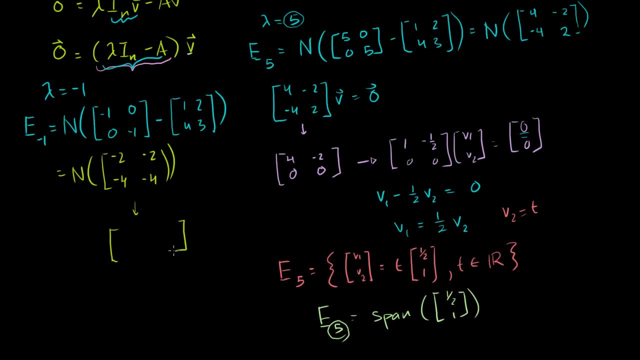 So if I replace my second row with my second row, plus 2 times my first row, So I'll keep the first row the same, minus 2,, minus 2.. And then my second row, I'll replace it with it, plus 2 times. 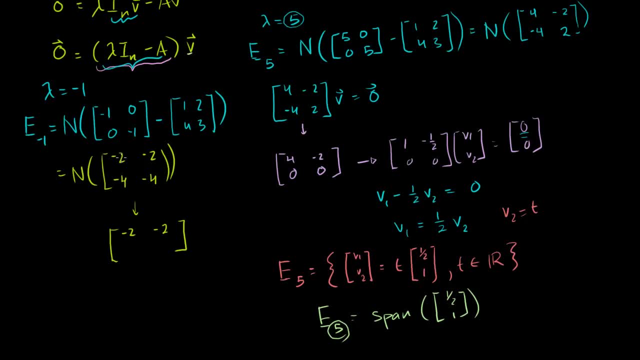 the first, or even better, I'm going to replace it with it plus minus 2 times the first. So minus 4 plus 4 is 0.. Minus 4 plus 4 is 0.. And then, if I divide the top row by minus 2, the reduced row: 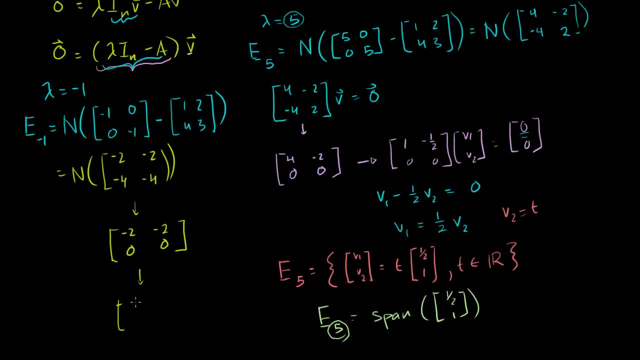 echelon form of this matrix right here, or this matrix right here is going to be 1, 1, 0. So the eigenspace that corresponds to the eigenvalue minus 1, is equal to the null space of this guy right here. 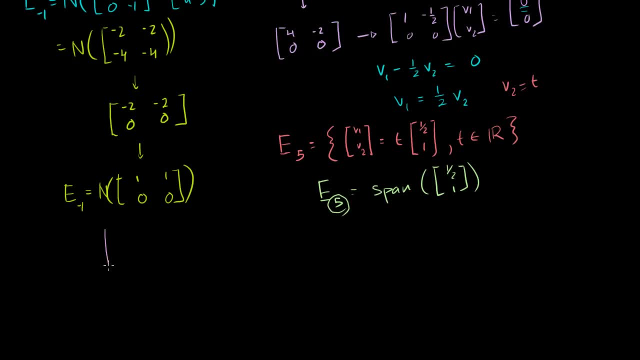 Or it's the set of vectors that satisfy this equation: 1, 1, 0, 0, 0. And then you have v1, v2 is equal to 0. Or you get v1 plus. these aren't vectors, these are just. 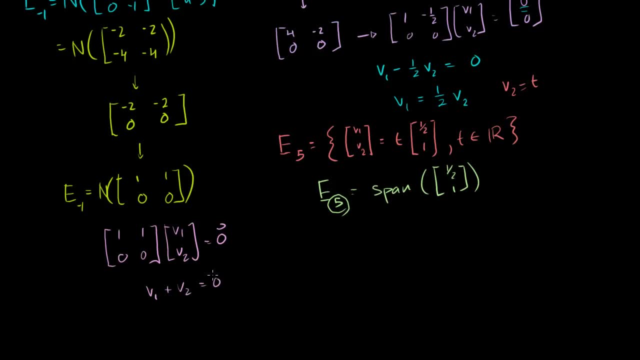 values. v1 plus v2 is equal to 0, because 0 is just equal to that thing, right there. So 1 times v1 plus 1 times v2 is going to be equal to that 0, right there. Or I could write: v1 is equal to minus v2.. 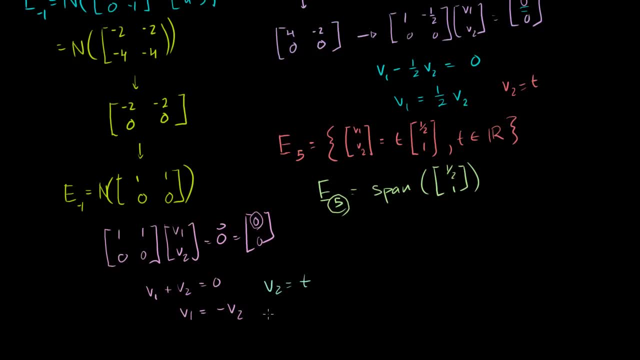 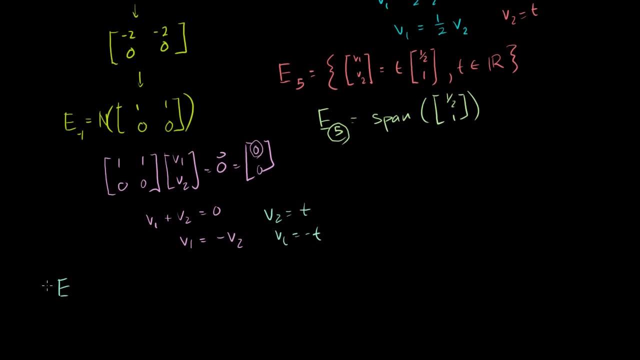 Or I could say that v2 is equal to t. we could say v1 is equal to minus t, Or we could say that the eigenspace for the eigenvalue minus 1 is equal to all of the vectors v1,, v2, that are: 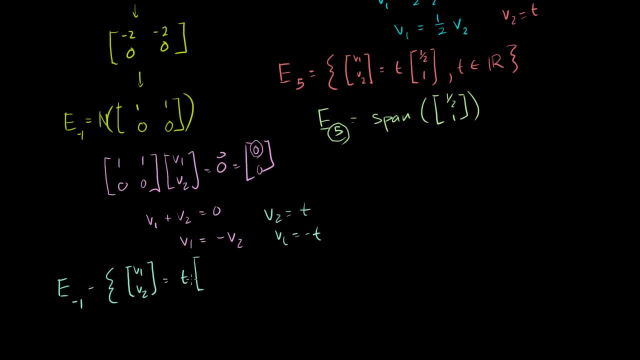 equal to some scalar t times. v1 is minus t and v2 is plus t. Or you could say this is equal to the span. This is equal to the span of the vector minus 1 and 1.. So let's just graph this a little bit, just to understand. 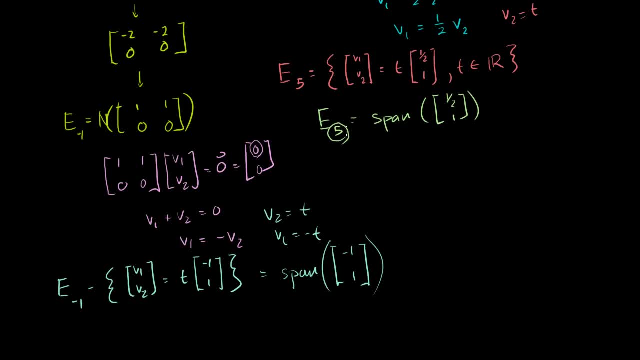 what we just did. We were able to find two eigenvalues for this: 5 and minus 1.. And we were able to find all of the vectors that are essentially, or we were able to find the set of vectors that are the eigenvectors that correspond to each of these. 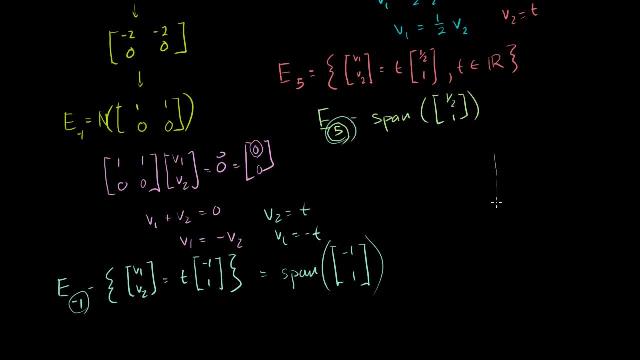 eigenvalues, So let's graph them. So, if we go to r2, let me draw my axis. this is my vertical axis, That's my vector, This is my horizontal axis. So all of the vectors that correspond to lambda equal 5. 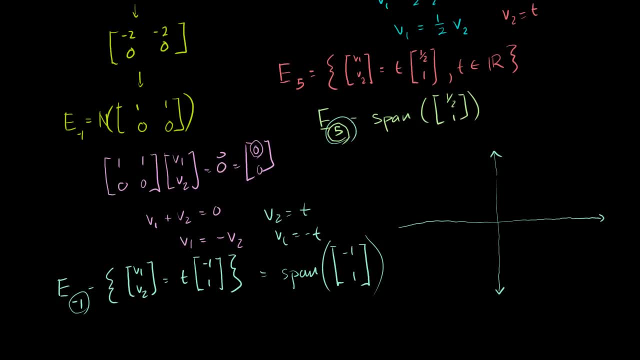 are along the line 1 half 1, or the span of 1 half 1.. So that is 1.. So you go 1 half and 1, just like that. So that's that vector, the spanning vector, But anything along the span of this, all the multiples of. 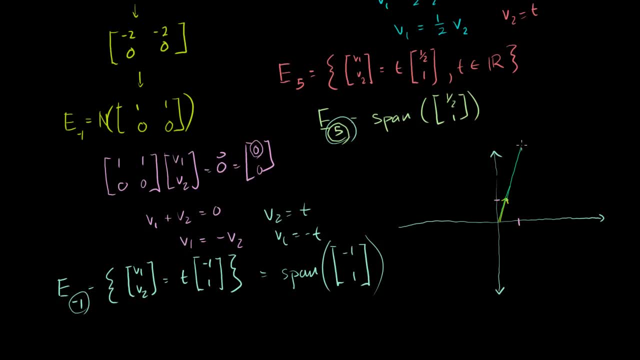 this are going to be valid eigenvectors. Anything along that line, all of the vectors, when you draw them in standard position, point to a point on that line. All of these vectors, any vector on there, is going to be a valid eigenvector and the corresponding eigenvalue is. 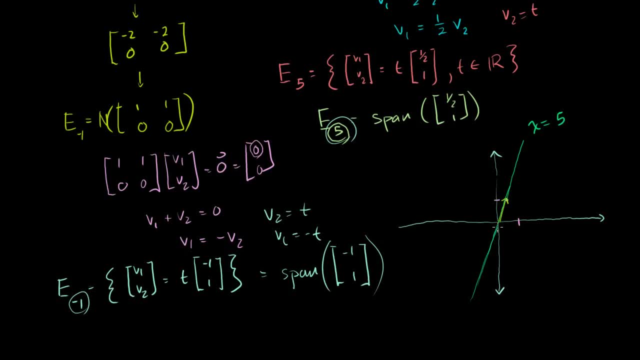 going to be equal to 5.. So you give me this guy right here. when you apply the transformation, it's going to be 5 times this guy You give me. if this guy is x, t of x is going to be 5 times. 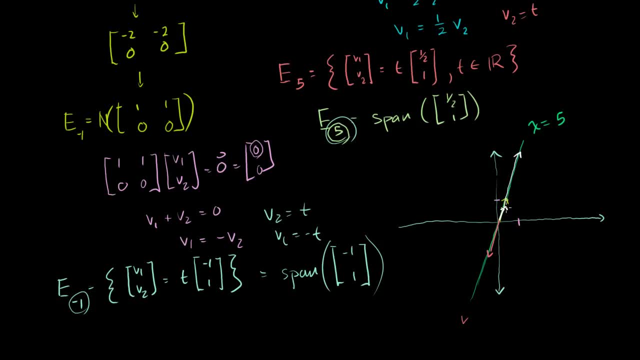 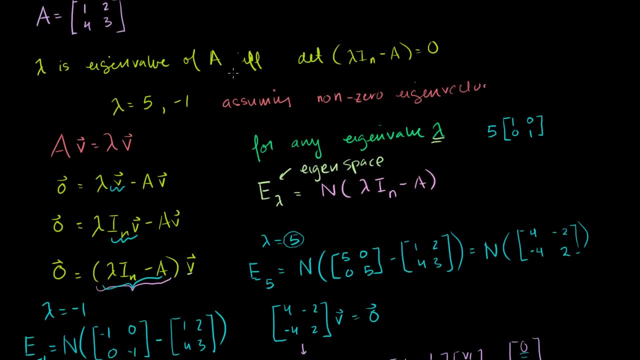 this guy. Whatever vector you give along this line, the transformation of that guy- and the transformation is literally multiplying it by the matrix A. Where did I have the matrix A? The matrix A right up there. You're essentially just scaling this guy by 5 in either. 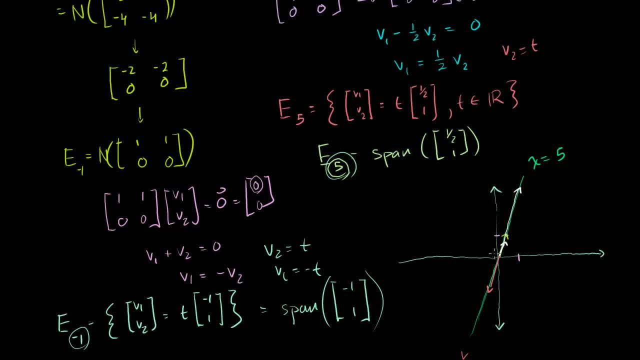 direction. This is for lambda equal 5.. And for lambda equals 1, it's the span of this vector which is minus 1, minus 1, 1, which looks like this. So this vector looks like that, But we care about the span of it. 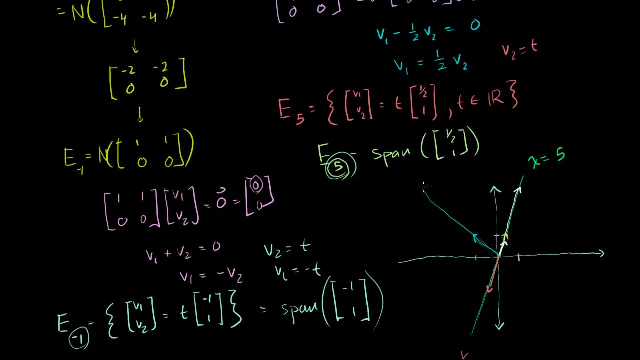 So anything, any vector in this set, any vector that when you draw in standard position, lies or points to points on this line, will be an eigenvector for the eigenvalue minus 1.. So lambda equals minus 1.. So if you take, let's say you take- the spanning vector here, 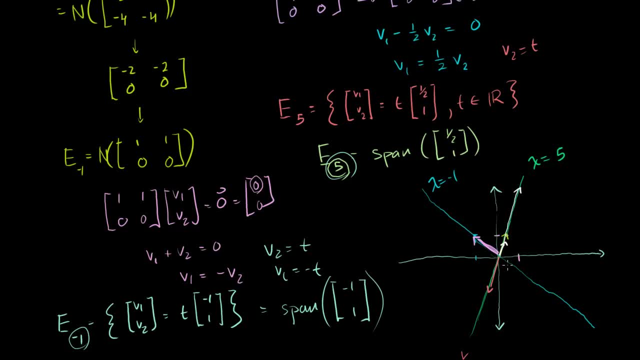 you apply the transformation, you're going to get minus 1 times it. So if this is x, the transformation of x is going to be that right there, Same length, just in the opposite direction. If you have this guy right here, you apply the.